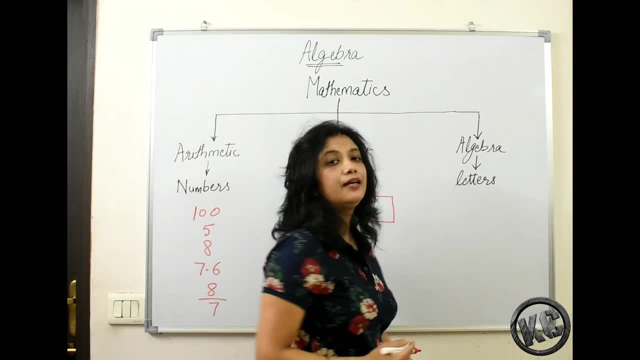 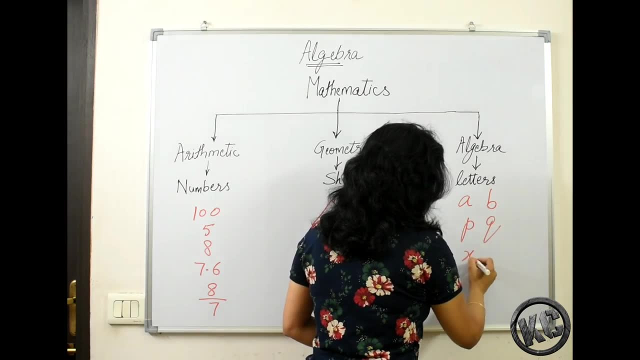 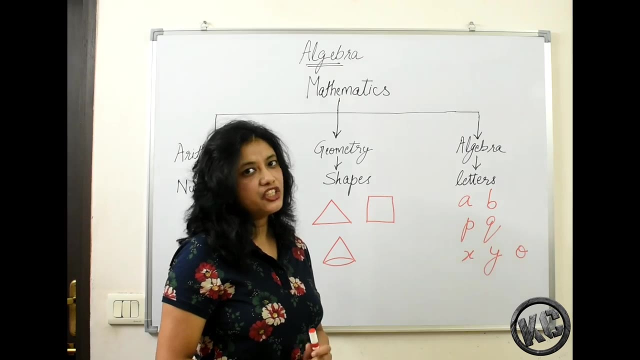 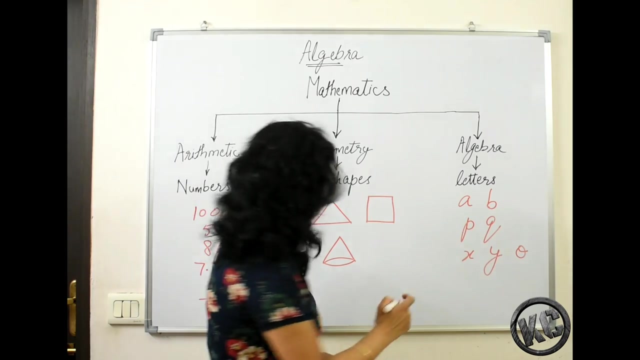 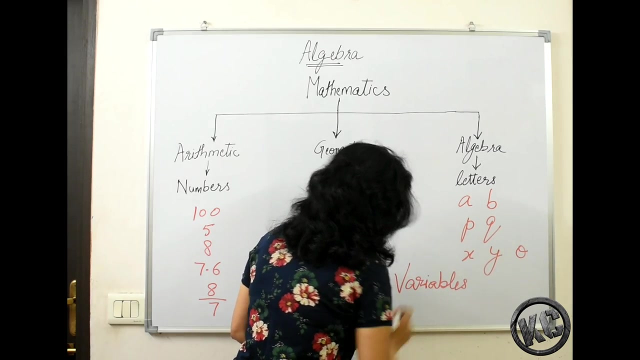 is algebra. In algebra we deal with letters, Letters like A, B, P, Q, X, Y, O, L. all these are letters of the English alphabet. They come under algebra. Now, these letters which we use in algebra are called variables. Now, why are these alphabets, these letters? why? 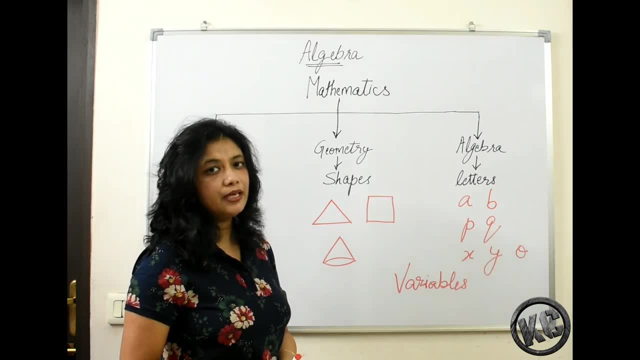 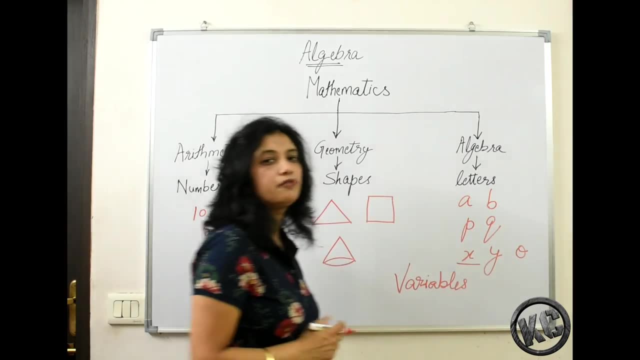 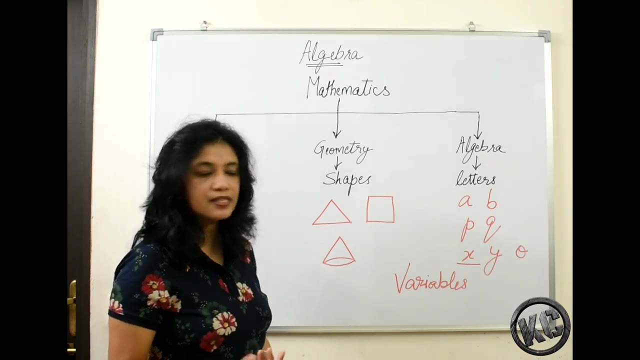 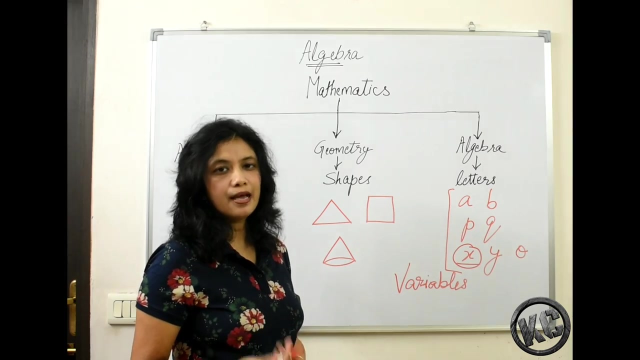 are these called variables? Because their value keeps varying, They don't have any fixed value. We cannot say that X has a value of 5 or 100 or 2000 or 6, because the values of all these variables, they keep varying with different sums. In one sum the value may be. 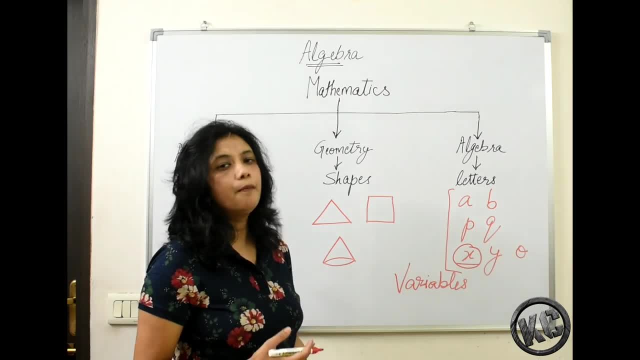 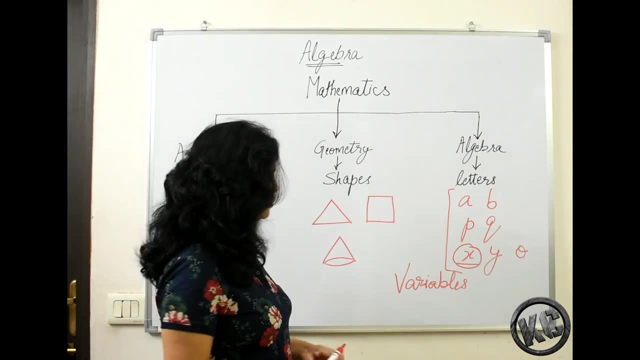 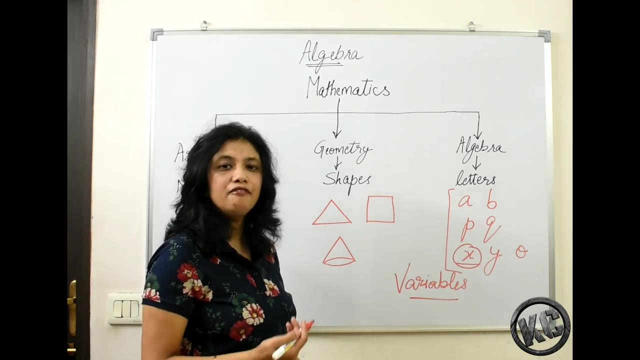 5,. in another sum the value of X may be minus 6.. So the values of these variables, they keep changing according to the problem sums. So therefore they are called variables. So all the letters in the English alphabet, they are under variables. Let us see how variables 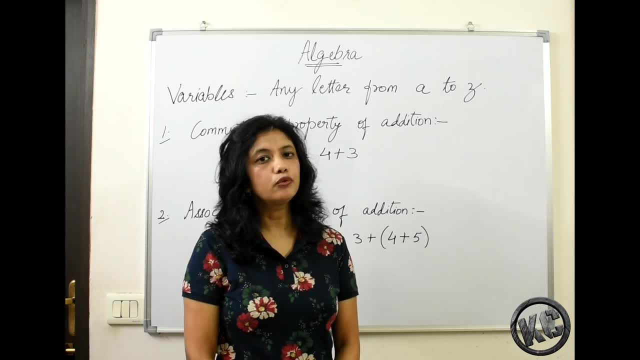 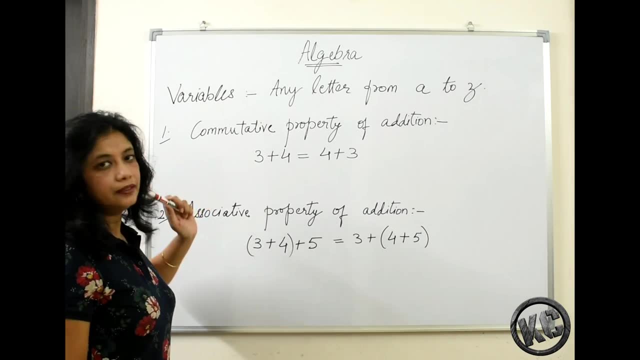 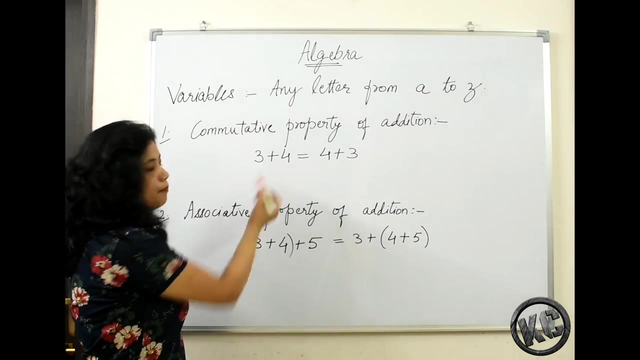 are useful to us. First of all, they help us to write rules and formulas in a general way. See, like you have studied earlier, the commutative property of addition. What does this property states That you can add any two whole numbers in any order. their sum remains the same. 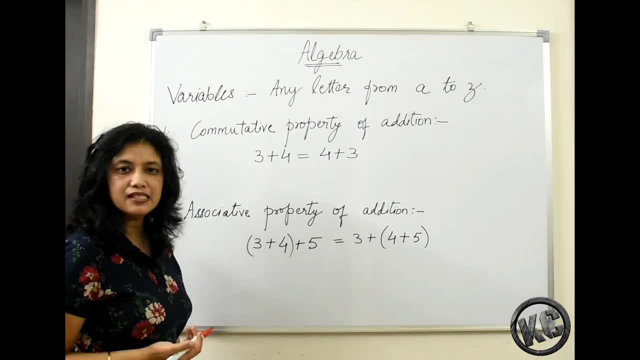 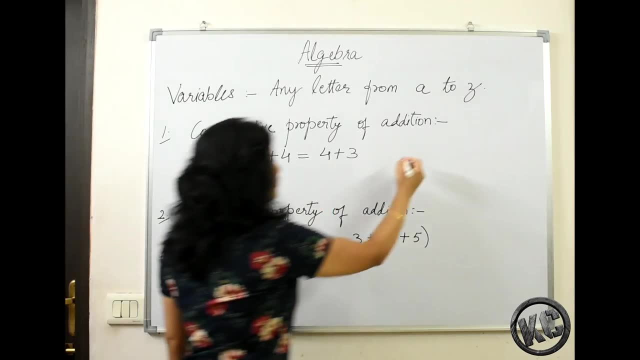 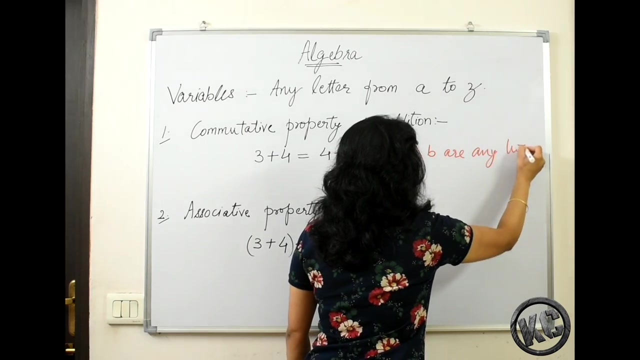 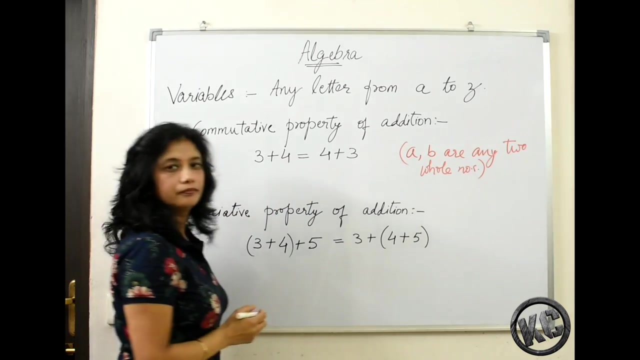 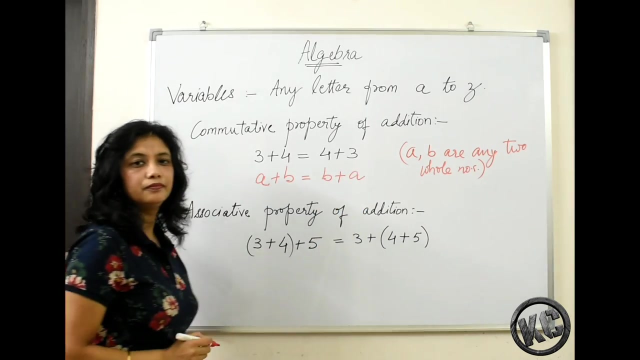 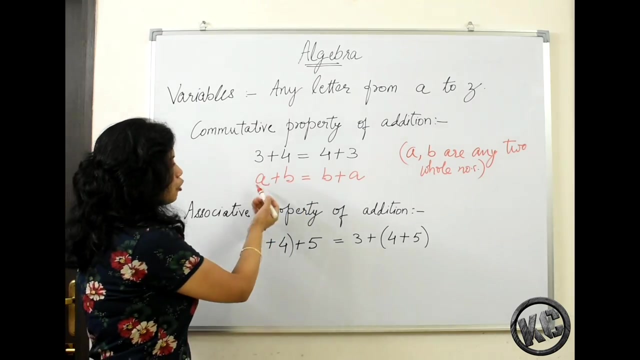 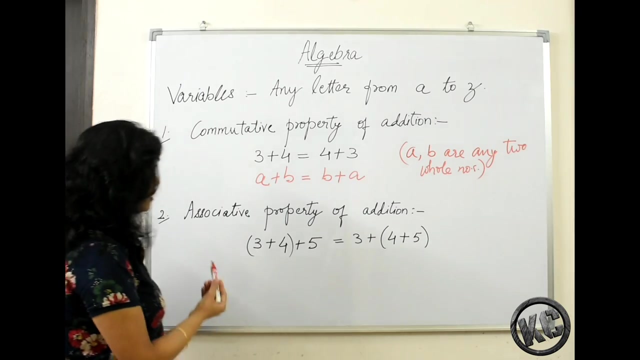 If you add 3 plus 4 or 4 plus 3, the answer will be same. So you can generalize this property using variable. We can generalize it in this way: Where A and B are any two whole numbers, Instead of A and B, you can write any two whole numbers and you can solve the property Now in the 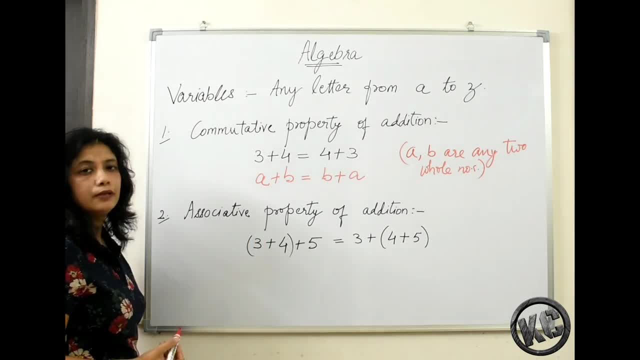 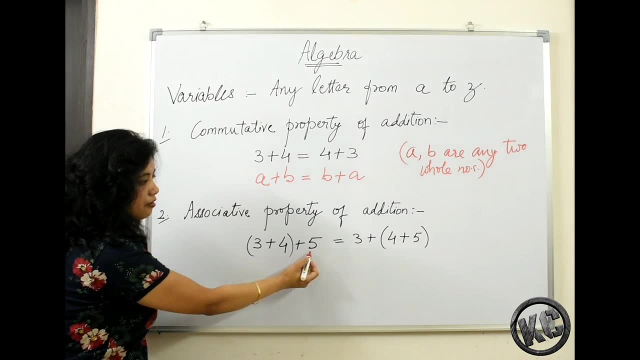 same way, associative property of addition is also true. Like 3 plus 4 plus 5, this can be written 3 plus 4. you can add first, then 5, or you can add 4 plus 5 and then 5.. So you: 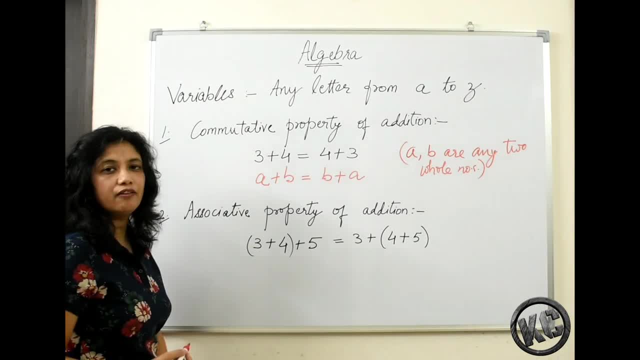 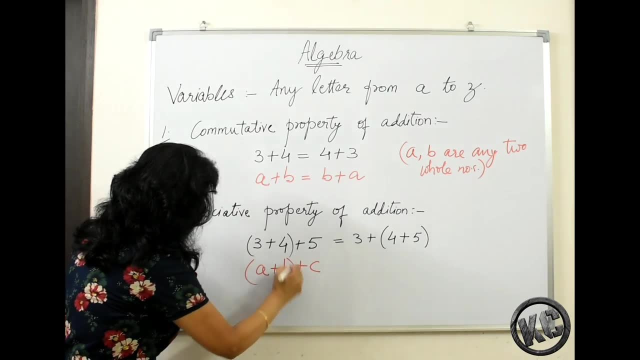 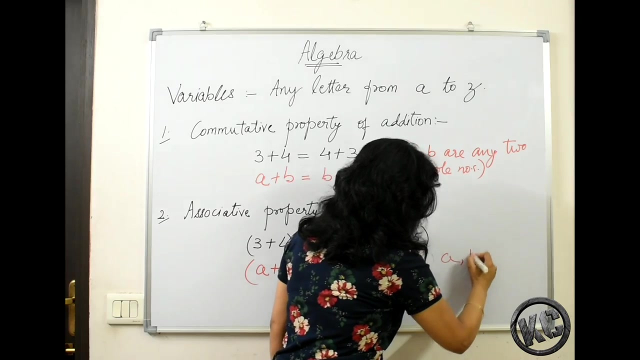 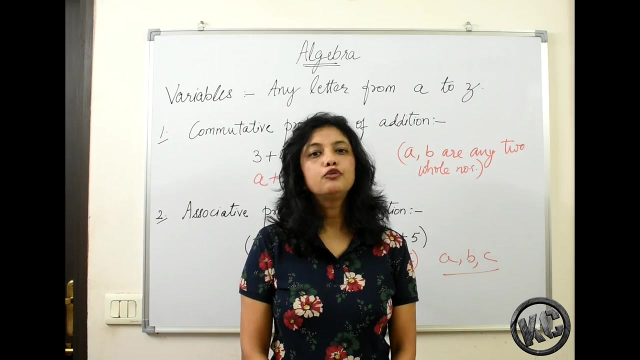 can add the sum to 3.. This also you can generalize using variables Like this: A plus B plus C, they are three whole numbers. You can write it like this: Where A, B and C are any three whole numbers? Another use of variable is to find the value of the unknown thing. We 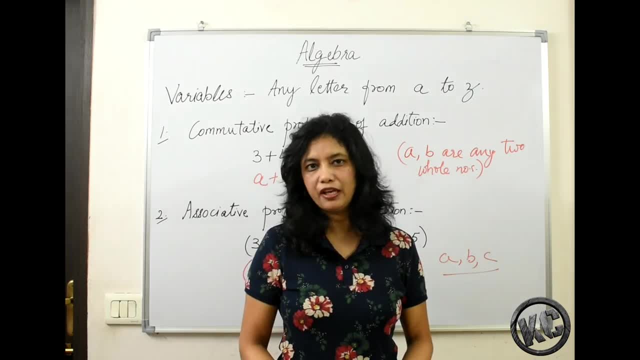 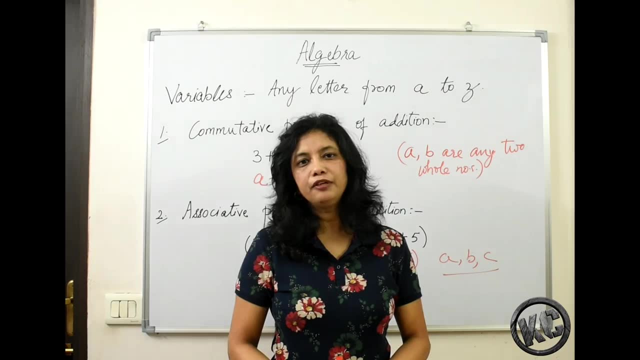 suppose that the value of the unknown is zero, So it is zero. So we can write any three whole unknown thing to be any of the variable, Any variable from the English alphabet, Any letter from the English alphabet we can assume as the variable and we find the solution to that. 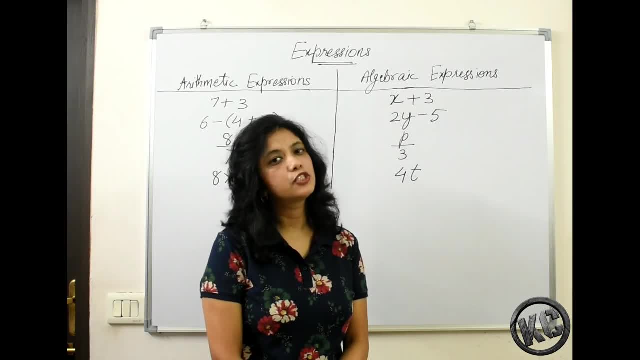 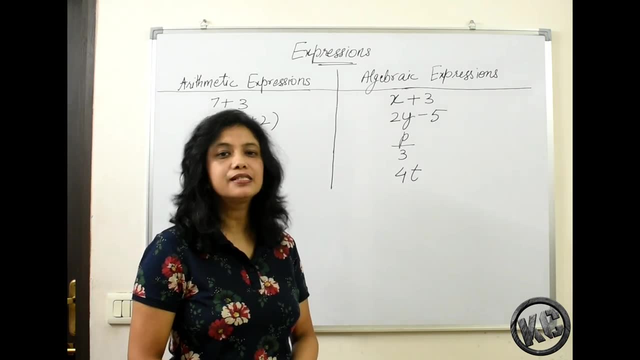 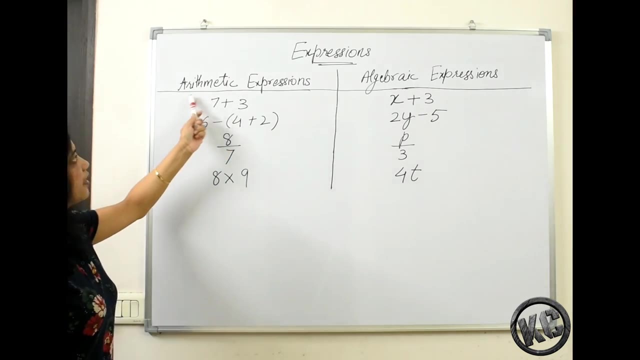 problem. Now let us study about expressions. See, we form expressions by using all the four number operations: Addition, subtraction, multiplication and division. Let us see how, See. we have two types of expressions: Arithmetic expressions and algebraic expressions. In arithmetic expression we use numbers and all the four operators, Means: plus, minus, multiplication. 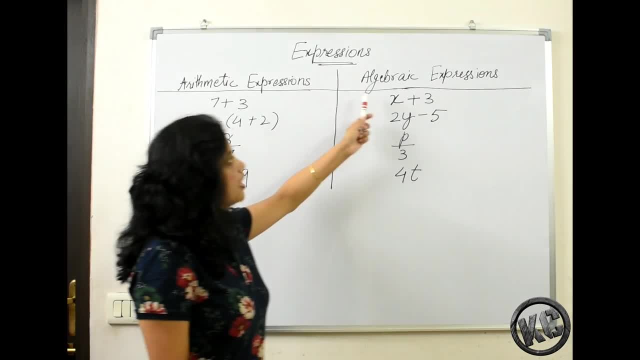 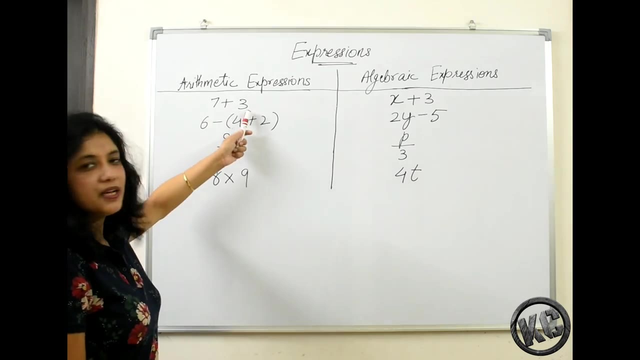 and division. they are called operators. Now in algebraic expressions we use variables. These are also called expressions with variables. We use variables, numbers and all the four operators. Now in algebraic expressions we use variables. These are also the four operators. See here: This is 7 plus 3. These all they have only numbers, 7 plus. 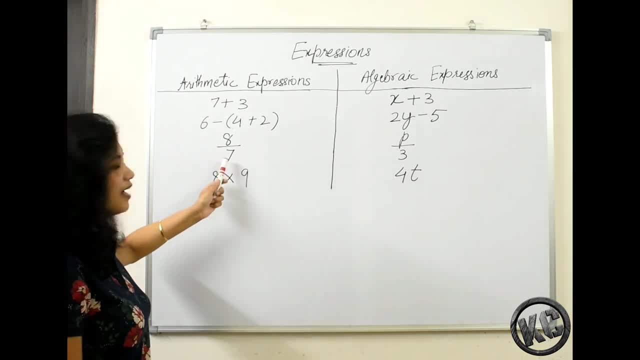 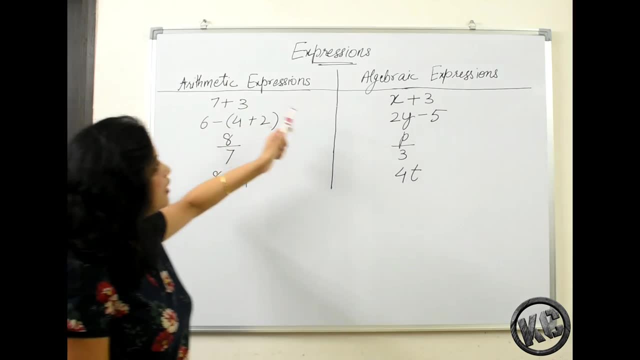 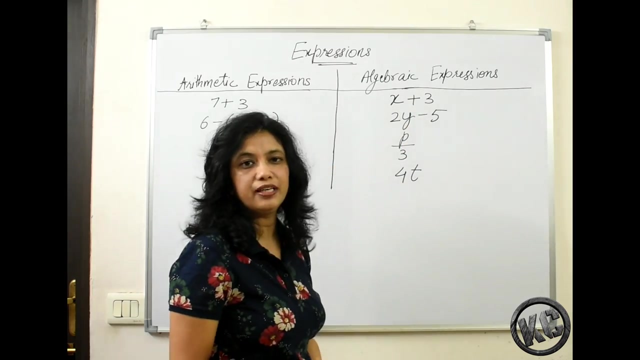 3, 6 minus 4 plus 2, 8 divided by 7, 8 multiplied by 9.. These are all arithmetic expressions. Now let us come to algebraic expressions or expressions with variables. See here This is read as x plus 3.. This is x plus 3, means x added to 3.. This can also be written like: